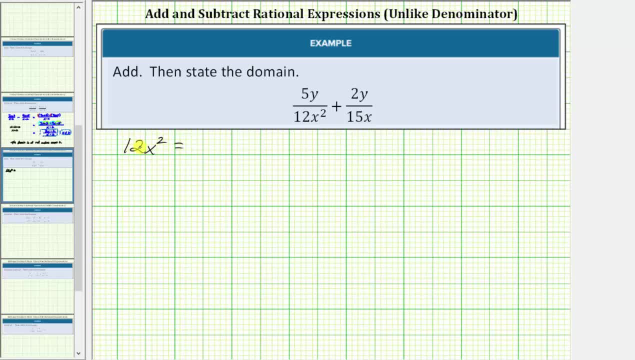 The prime factorization of twelve is two times two times three. So we'll write twelve x squared as two times two times three times x times x. And then for fifteen x, because the prime factorization of fifteen is three times five, we'll write fifteen x as three times five. 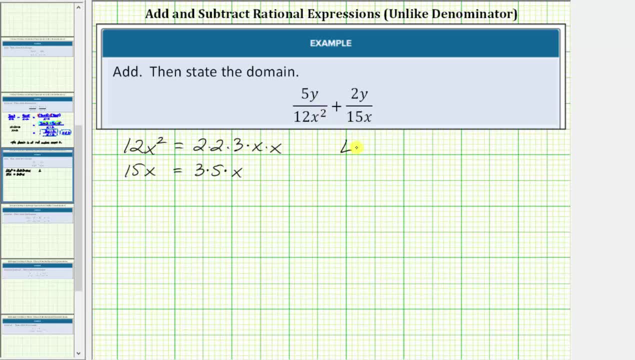 times x. And now let's build the least common denominator. To begin, the least common denominator must contain all of the factors of the first denominator And therefore the LCD must contain two factors of two, a factor of three and a factor of two. 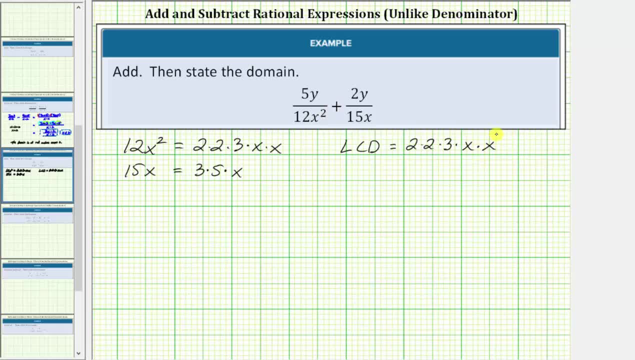 And two factors of x. And now, looking at the second denominator, let's see if any of these factors are missing from the LCD. Notice. we already have a factor of three, We also have a factor of x, But we don't have a factor of five listed in the LCD. 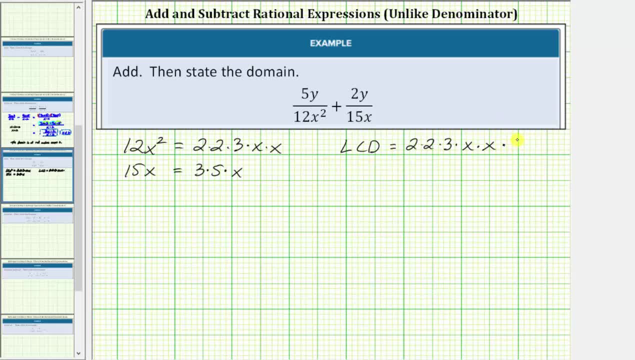 Which means we need a factor of five in the LCD Notice. now all the factors of both denominators are listed in the LCD. So this product is the least common denominator. Well, two times two times three times x is the least common denominator. So we have: three times five is equal to sixty. 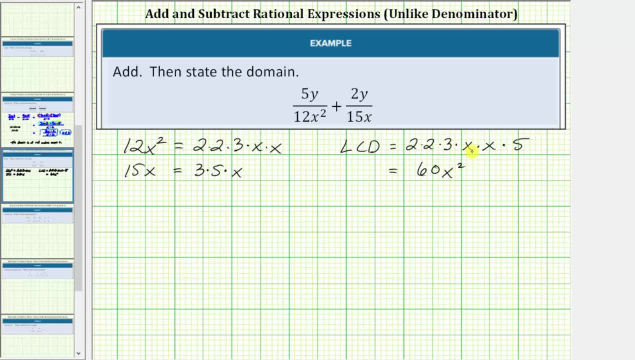 And therefore the LCD is sixty x squared. For the next step, we'll write both fractions as equivalent fractions with the denominator of sixty x squared. So to begin, we have five y divided by twelve x squared, plus two y divided by fifteen x. Looking at the first fraction to write an equivalent fraction. 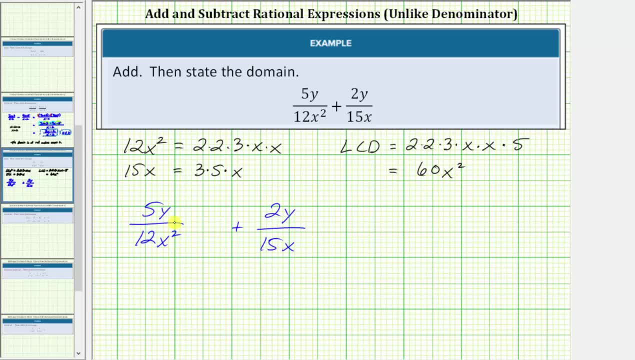 with the denominator of sixty x squared, we need to multiply the numerator and denominator by five, Because twelve x squared times five is sixty x squared. Now, looking at the second fraction, to write an equivalent fraction with the denominator of sixty x squared, we need to multiply. 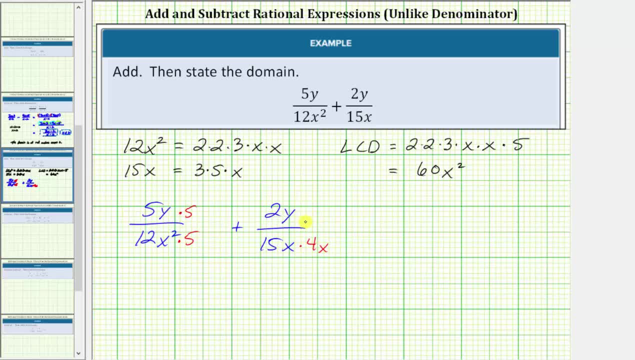 the numerator and denominator by four x, Because fifteen x times four x equals sixty x squared. Notice now: both denominators are sixty x squared. So now we can add the numerators. Here we have twenty five y plus this would be eight x y.